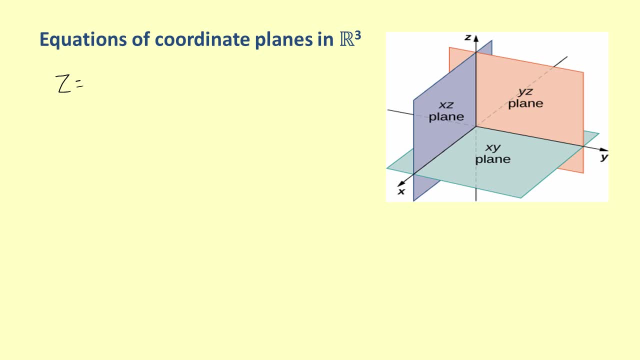 Let's think about the equation z equals 0. in three-dimensional space, We are not given any restrictions on x or y, so all points- x, y, z- with a coordinate of zero satisfy this equation. Therefore, the equation z equals 0 defines the x- y plane In a similar manner. 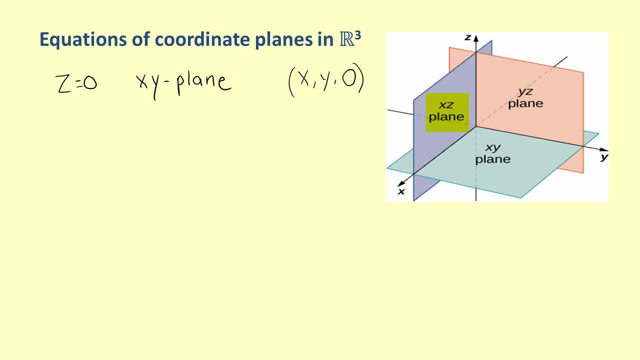 the x z plane is described by all points having a y coordinate of zero. thus, the equation y equals zero defines the x z plane. Likewise, the y z plane is described by all points, all points having an x coordinate of 0. Thus, the equation x equals 0 defines the y z plane. 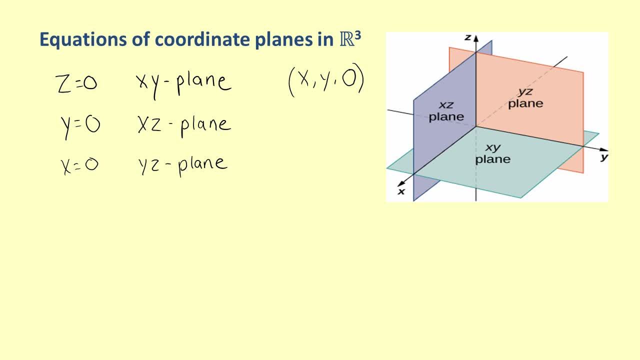 Now suppose we want to describe a plane that is parallel to the x- z plane. Let's suppose this plane crosses the y axis at a y coordinate of b. How would we describe this plane? Well, its y coordinate is always b, while its x and z coordinates can be any value, That is. 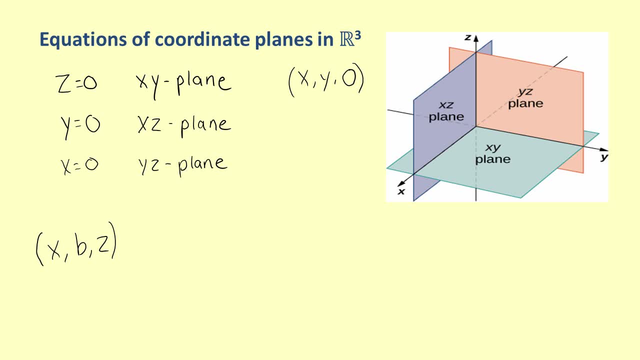 any point x, b, z will be on the plane. So we can see that the equation y equals b will describe a plane parallel to the x- z plane and having a y coordinate of b. Similarly, a plane parallel to the x- y plane crossing the z axis at a value c will be defined by: 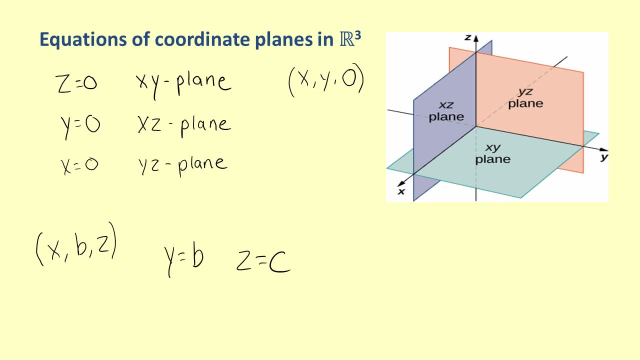 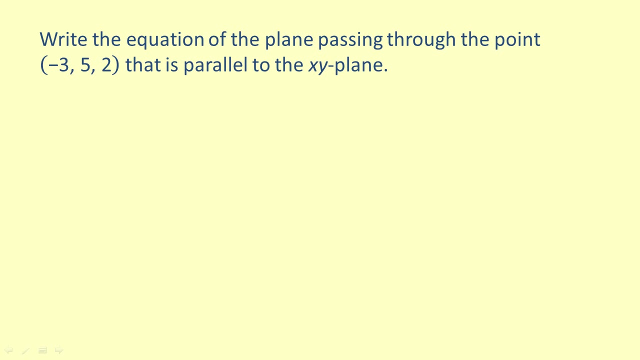 the equation z equals c, And a plane parallel to the y- z plane crossing the x axis at a value a will be defined by the equation x equals a. This problem asks us to write an equation for a plane that is parallel to the x- y plane and that also passes through the 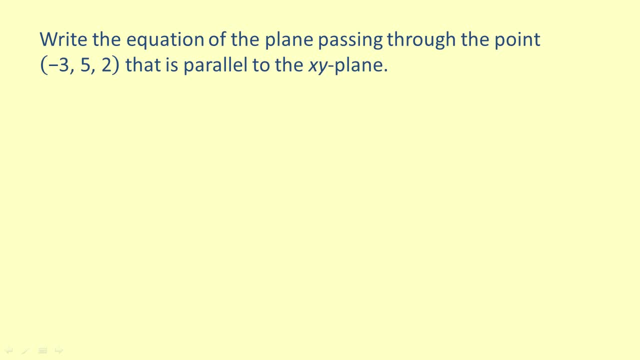 point. We know that the x- y plane is the plane where the x and y coordinates can be any real number, while the z coordinate is fixed at 0. Therefore, the plane we are looking for is a plane where the x and y coordinates can again be any real number.